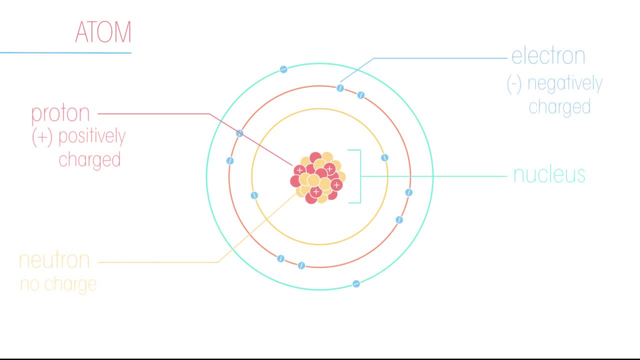 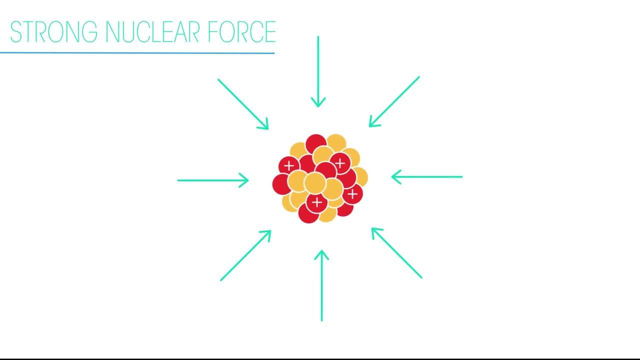 nucleus. For more information on atomic structure, watch this video. A strong nuclear force holds the positive protons and neutral neutrons together in the nucleus and is what determines if a nucleus is stable. In stable nuclei, the force is strong enough and brings sufficient energy to hold the nucleus. 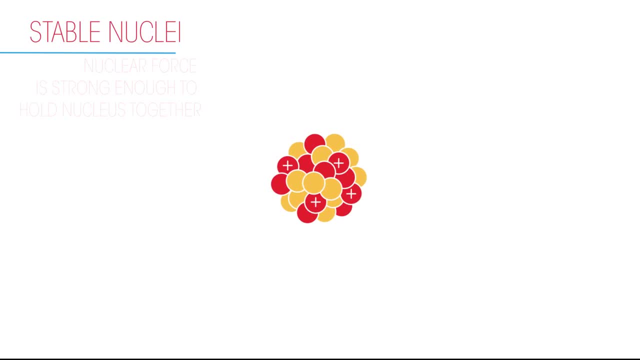 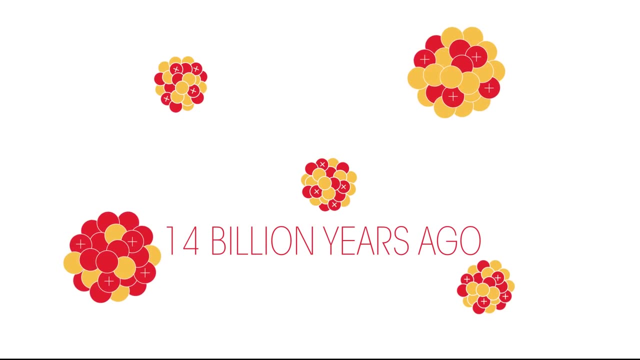 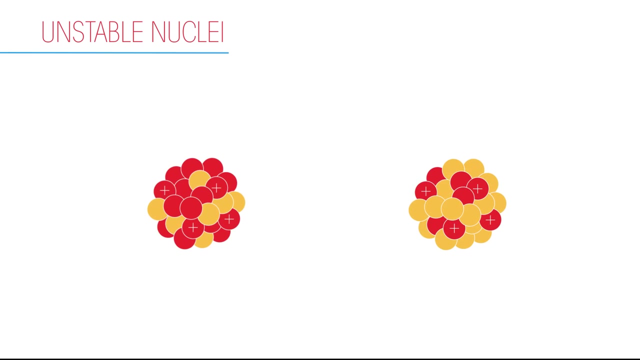 together permanently. Most of the nuclei formed during the Big Bang nearly 14 billion years ago are still in existence today. But not all nuclei are stable. Unstable nuclei either have too many protons or too many neutrons, upsetting the strong nuclear forces. Unstable nuclei try to balance themselves by giving off the excess. 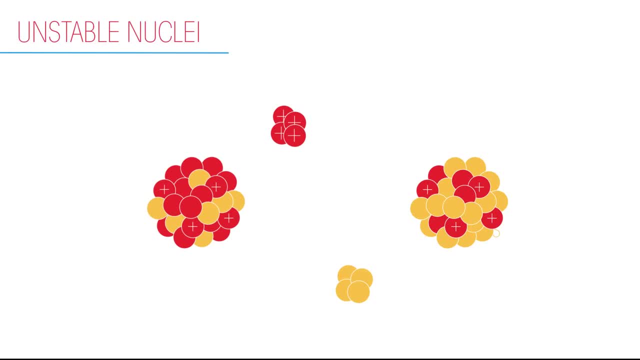 proton or neutron. This is radioactive decay. Unstable nuclei are radioactive and emit radiation. There are three types of decay: Alpha decay, beta decay minus or beta decay plus. Alpha decay is the loss of an alpha particle. An alpha particle is made of two neutrons and two protons. 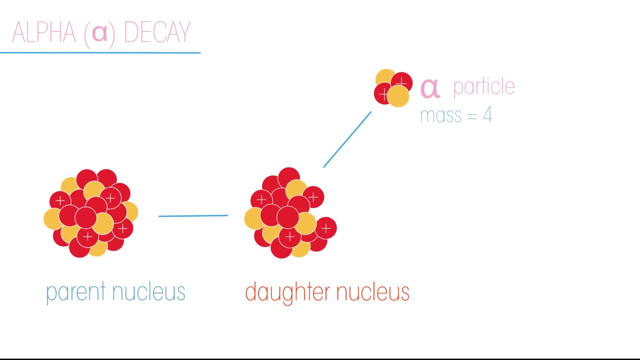 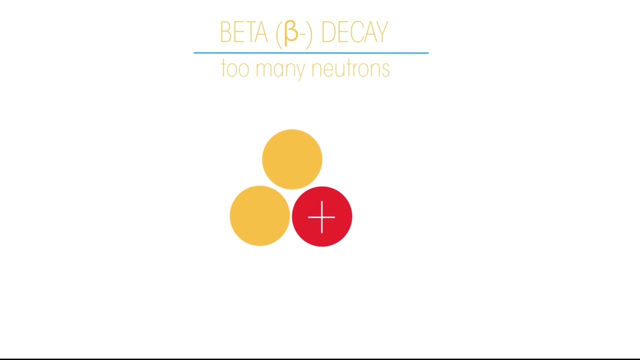 They have a mass of four and a charge of one. When an atom loses an alpha particle, the mass number decreases by four and the atomic number decreases by two. A new element is formed that is two places lower in the periodic table. When an isotope has too many neutrons, it decays. 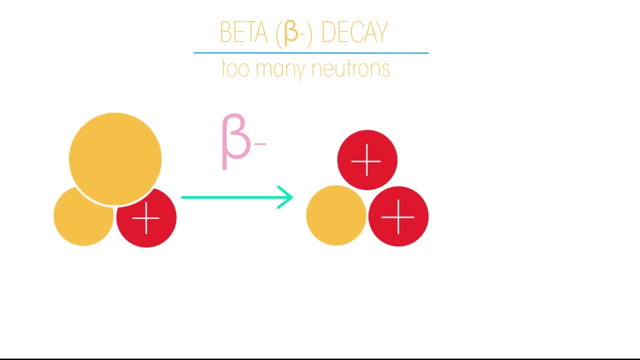 by beta minus decay, A neutron changes into a proton and an electron. The proton is retained by the atom while the electron is lost. The lost electron is high energy and is called a beta particle. By losing a neutron whilst gaining a proton, the mass number of the atom 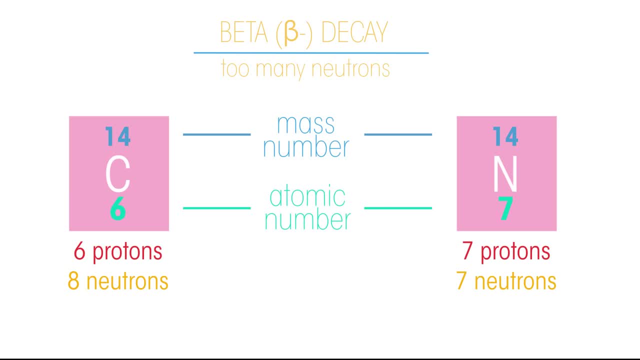 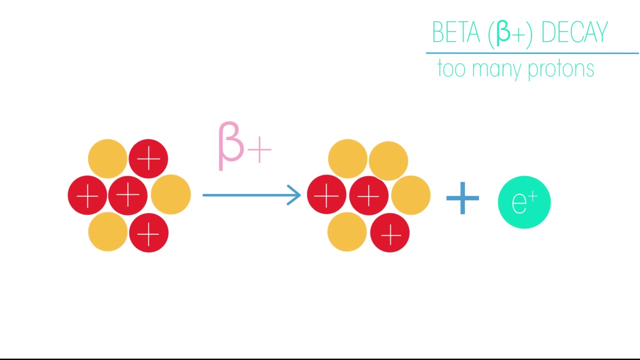 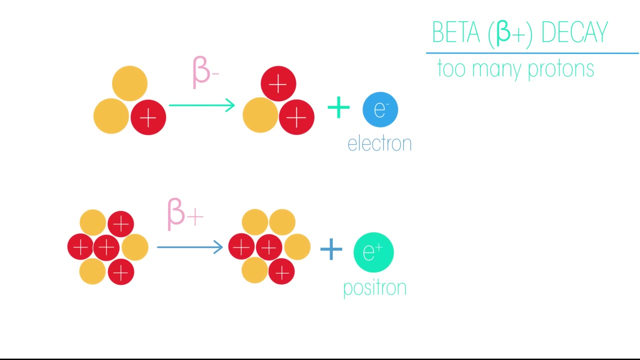 remains the same, but the atomic number increases by one. A new element is formed that is one place higher in the periodic table. When an isotope has too many protons, it decays by beta plus decay. A proton is converted into a neutron and a positive beta particle called a positron.